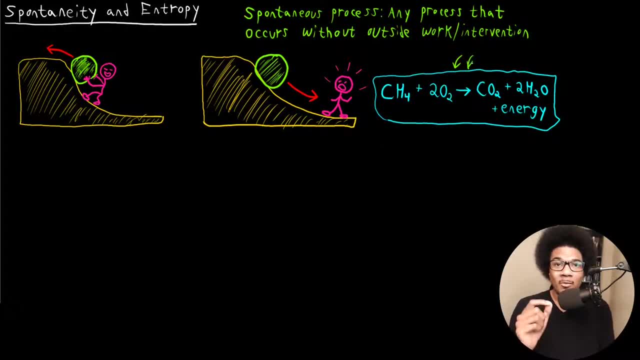 that were covered in the previous course. but those tools are very limited in their scope. They can really only answer the question of energy flow- Is energy going into or out of my system? More or less like an energy bookkeeping type of thing. But what it really doesn't address 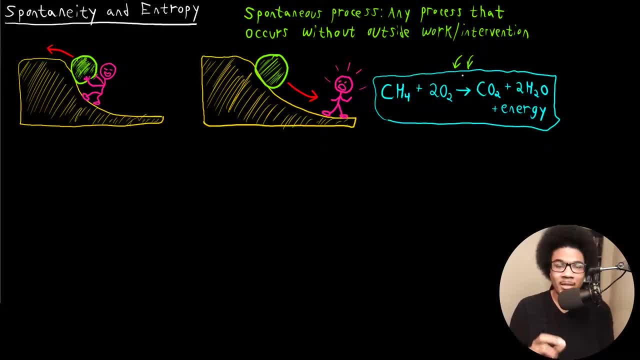 what just using the first law of thermodynamics and enthalpy does not address is why this reaction proceeds in this direction in the first place, right? Why does it proceed in this direction and not the opposite direction? Can it proceed in the opposite direction? How? 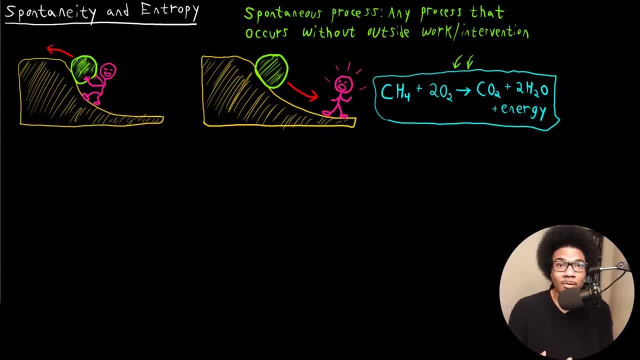 likely is that Those are things that you can answer with energy and thermodynamics, but not with the current understanding that we have, with just the first law of thermodynamics and just an understanding of enthalpy. So we'll have to broaden our understanding of 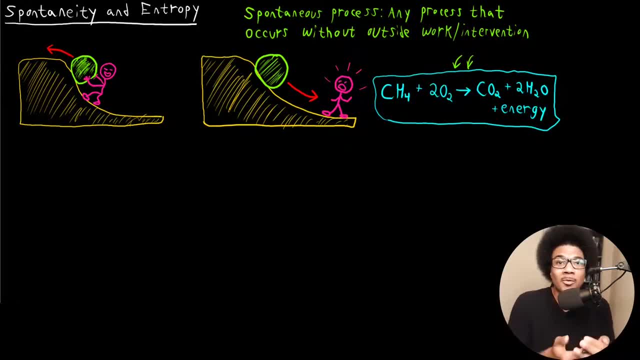 thermodynamics, before we're able to answer questions of why do certain reactions have a reaction, Why do certain reactions happen in the first place, right Or be able to predict is a reaction likely to occur right? And so one of the key pieces in being able to predict whether 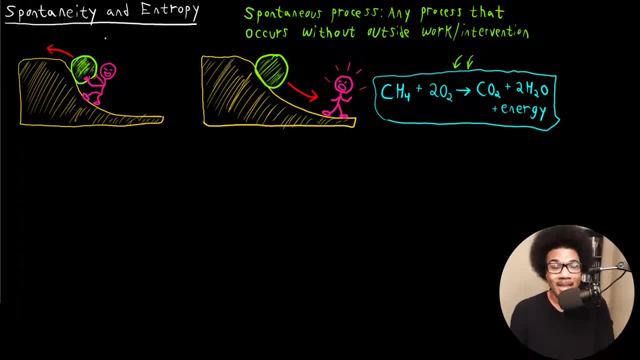 a reaction is likely to occur or not. is this concept of spontaneity? So spontaneity is based on spontaneous processes. So these are any processes that occur without any outside work or intervention, right, And I think the best way to kind of introduce this topic is just with some 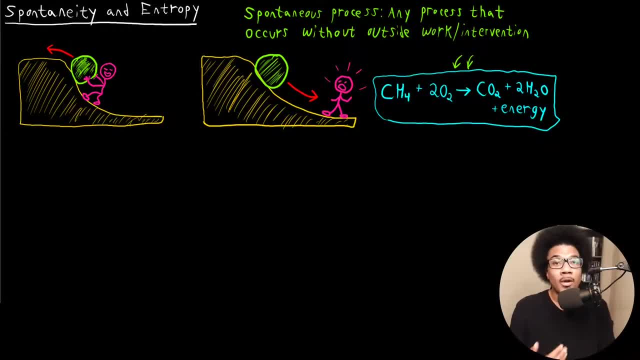 processes that we would describe as either spontaneous or non-spontaneous. So here on the left I've got a guy who is pushing a boulder up a ramp right. So he has this boulder and he's pushing the boulder up the ramp. Now, if this guy was not there pushing the boulder up the ramp, 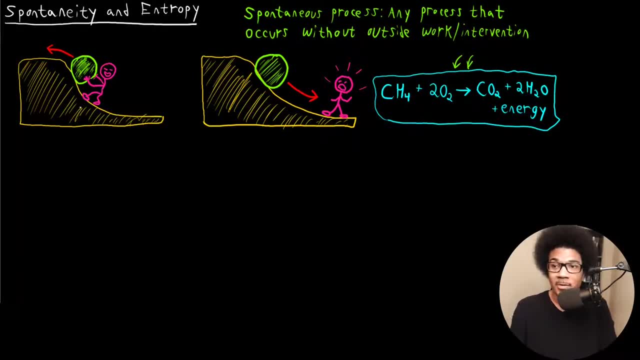 the boulder would not go up the ramp right? Very simple to understand. It requires work, right? He has to apply some force, right? Remember, work is some force applied over a distance, So he has to apply some force in order to move the boulder at all. 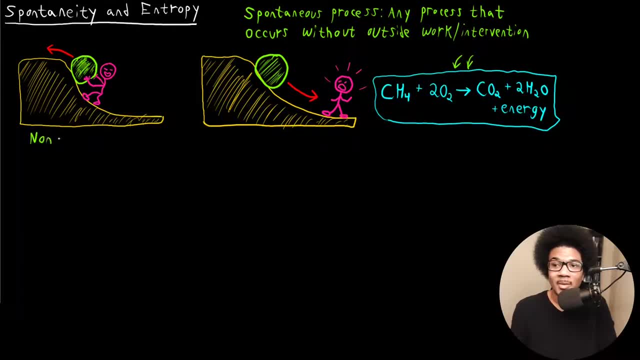 up this hill, right? So this is what we refer to as a non-spontaneous process, Right? Не-spontaneous? right? You take this guy out of the picture. the ball would not roll in this direction unless he was applying this applied force to move it up the ramp. 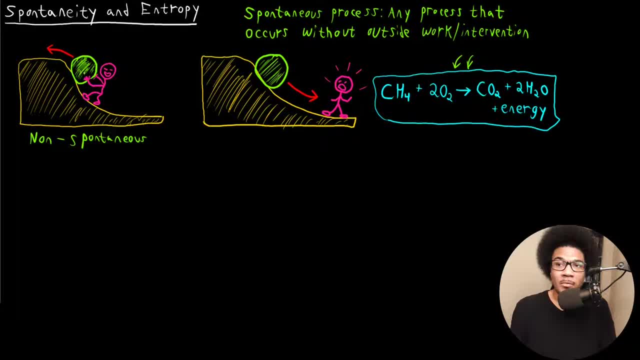 ék到 Now in the opposite case. right? so if we were just to take this guy and move him back down the ramp and leave the boulder where it was, then the boulder would move down this ramp without any assisted force. You wouldn't need anyone pushing on the opposite direction. 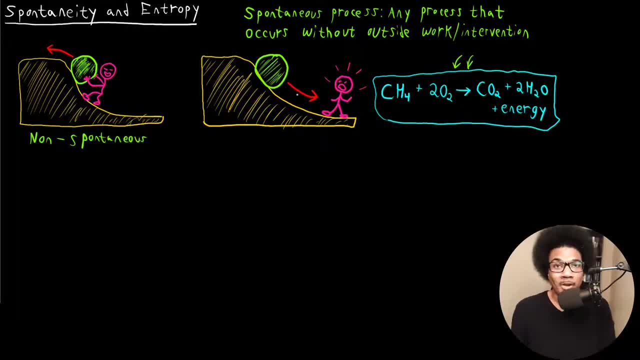 Since it's sitting on a downward incline, it would roll down this incline without any outside intervention or force. This is what we would call a spontaneous process, Right? so this would happen spontaneously until it hits the guy or rolls him over, right? 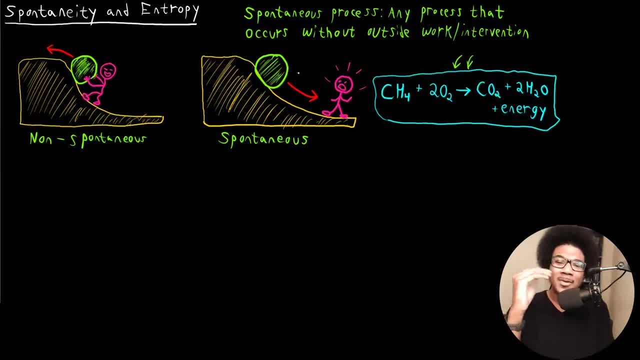 That's why I have him looking alarmed here, right? So yeah, so this is a spontaneous process, one that doesn't require any outside work or intervention. A non-spontaneous process is one that does require work or intervention, right, If you want to think about a chemical version of a spontaneous process, right, something? 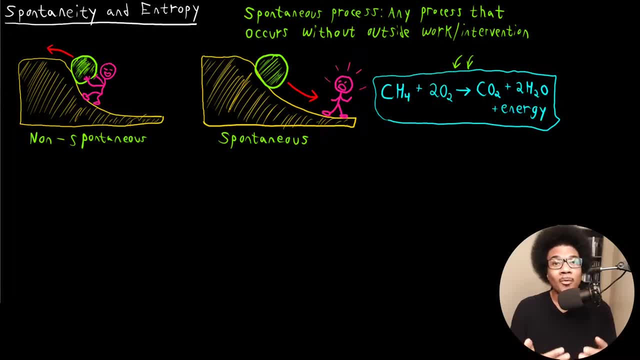 we may think about in chemistry. think about a chemical version of a spontaneous process. Think about iron rusting right? So if you leave iron outside, as it's naturally exposed to oxygen and moisture in the air, it is going to rust. Now, that's a process that takes a really long time to happen, but it is a spontaneous. 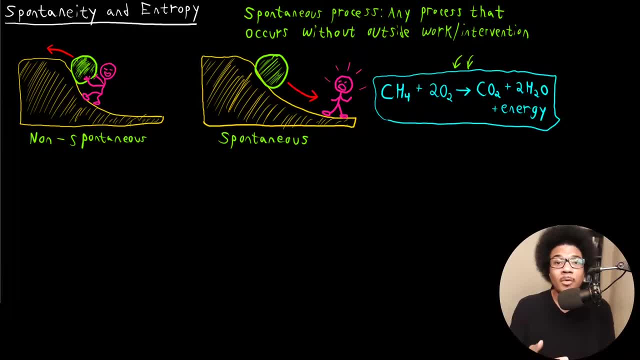 process. It's going to occur in that direction, right? So this brings up an interesting point about spontaneity. Saying that something is spontaneous in no way means that it's going to occur quickly, right. Spontaneous processes can be fast. 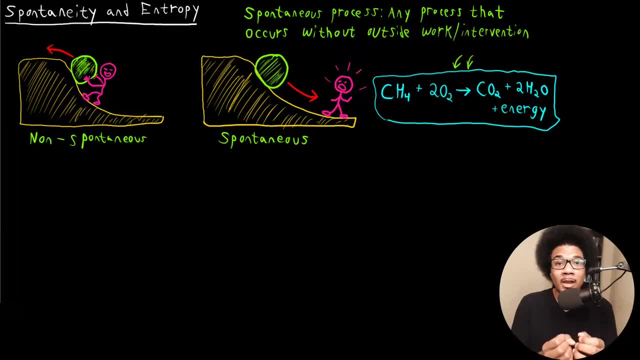 They can be slow. All we're really saying is that we are guaranteed. We are guaranteed that this process will occur with no outside intervention, force or energy. Now, a key thermodynamic property in order to figure out whether something is spontaneous or not is entropy right. 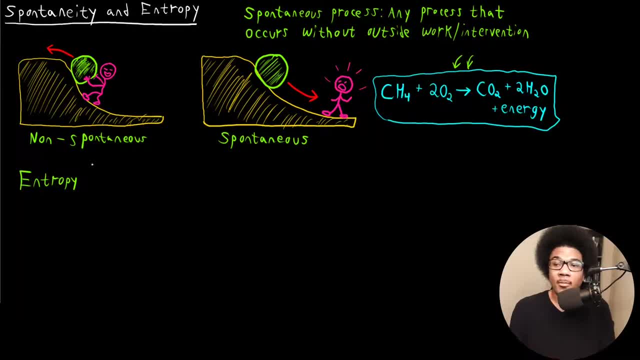 So entropy, and we use the variable a capital S to denote entropy, right, So we're going to go through. we're going to have a couple of different definitions for entropy And I'll give the mathematical definition in the video on the second law of thermodynamics. 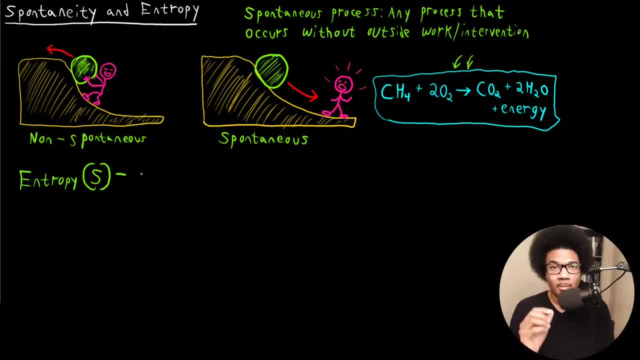 But for now, just think of entropy as a measure of molecular randomness or disorder. right, So this is a measure of molecular randomness or disorder. So you may have heard this definition used before in the past. right, It's, entropy is a measure of disorder, right? 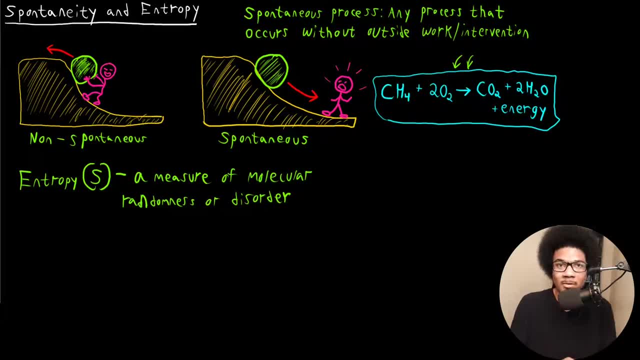 So everything is going to tend towards disorder. That's going to be the second law of thermodynamics, But you can think of entropy at this point just as a measure of molecular randomness or disorder, And it's going to be a key quantity for us in order to figure out whether a process is. 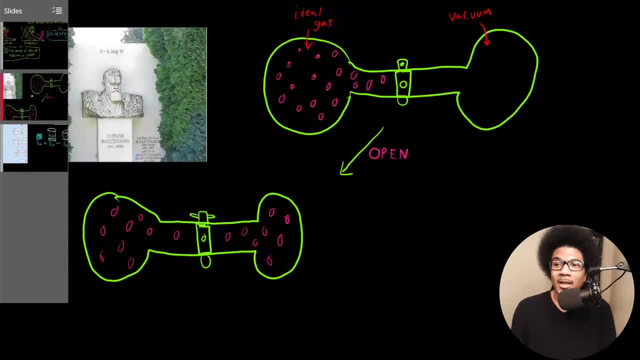 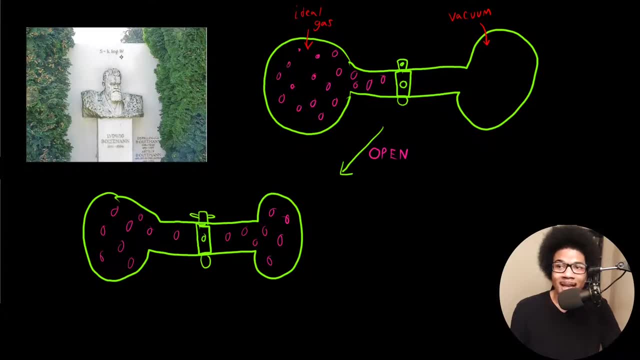 going to be spontaneous or not. Now, entropy is very important. In fact, it's so important that the guy who invented the equation for entropy has that equation nestled right above his gravestone. So this is the gravestone of Ludwig Boltzmann. 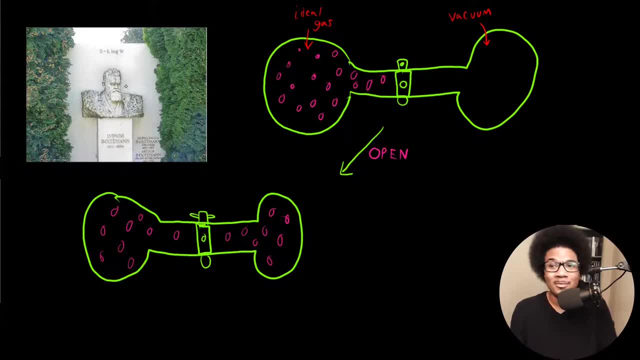 And if you've taken statistics or even some physics classes before, you've probably heard Boltzmann's name before. right, The Boltzmann constant. You know you've probably heard this before, but his biggest claim to fame was figuring out this equation for entropy which, if you can't see it, it says that the entropy is: 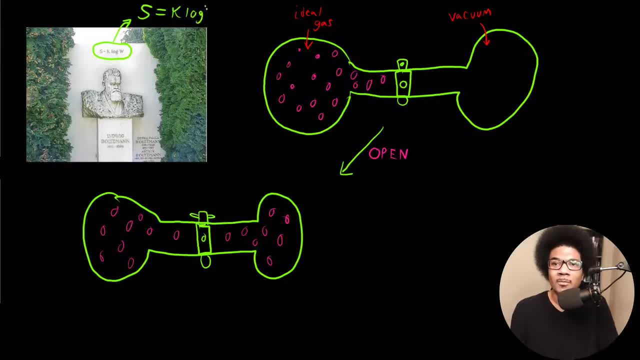 equal to K log W, where K is the Boltzmann constant and W is something known as the degeneracy. But you can kind of think of that W as just a measure of the randomness, right. So this entropy is going to be equal to this equation. 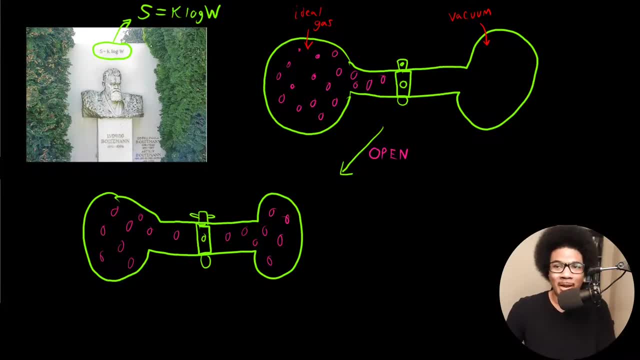 And it's so popular that it sits above his gravestone. OK, so we're going to make this link between entropy and spontaneity very explicit when we talk about the second law of thermodynamics. What I want to do for the rest of this video is just kind of give you a little bit of insight. 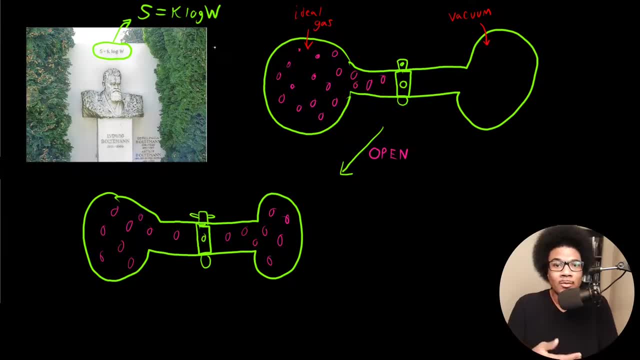 into how intuitive entropy is, into kind of discussing what processes are likely to occur, right? So let's think about this following example that I have drawn out here, right? So what I have here is a two bulb system that has like a stopcock in the middle. that you 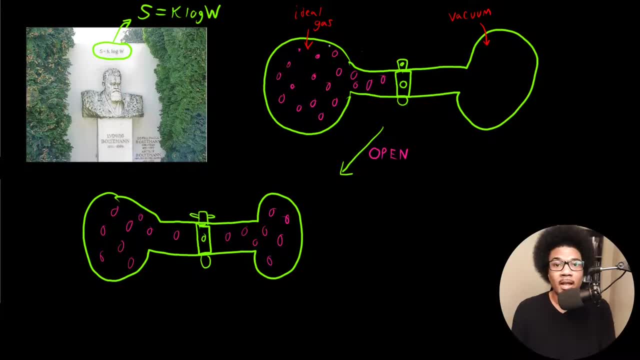 can turn to open or close respectively. right In this one I have an ideal gas on the left bulb And a vacuum on the right bulb right. So if you open this stopcock, then the gas is going to expand spontaneously, right? 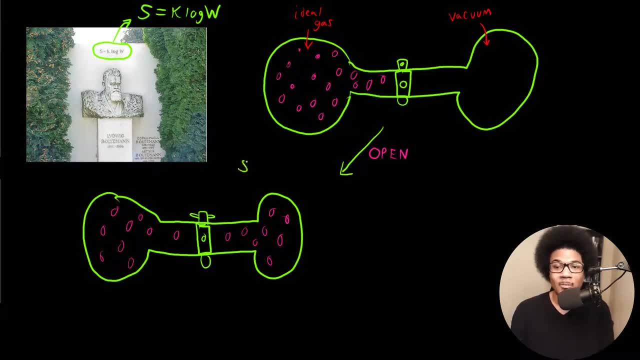 So this opening and expansion of the gas is going to be a spontaneous process, right? It won't require any outside work. There will not have to be any forcing or pushing of the gas into the other bulb. It is going to expand to the other bulb spontaneously, right? 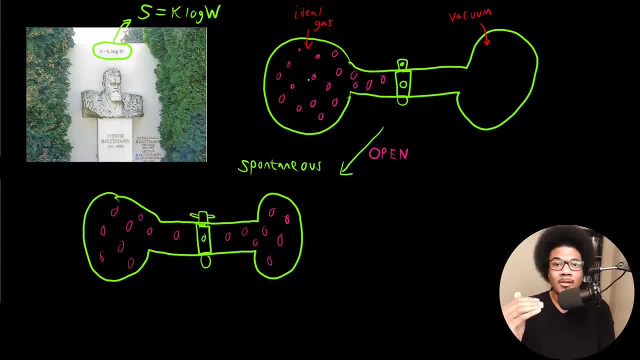 Gases will always expand to fill the other bulb Right The available volume spontaneously. And if you want to kind of think about it, think about it. What if we tried to go the opposite way, right? What if we tried to take this gas that's now expanded into the two bulbs and we wanted 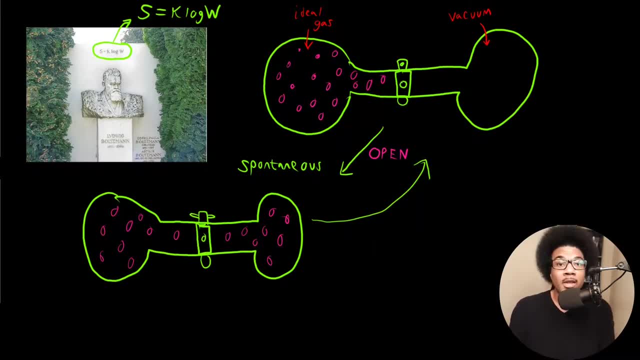 to return it to this original state. Well, we'd have to either evacuate some of the gas from this bulb, return this to vacuum, reclose the stopcock right. It's going to take a lot of energy and work in order to compress the gas back into a single. 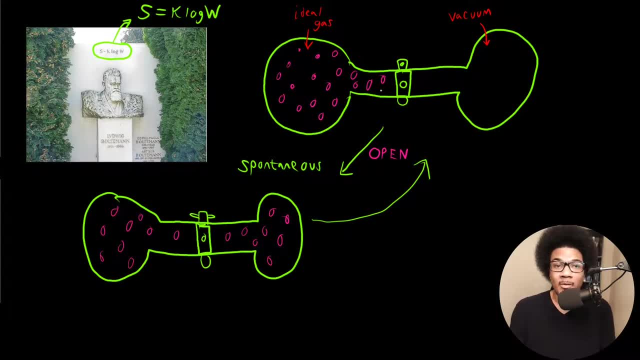 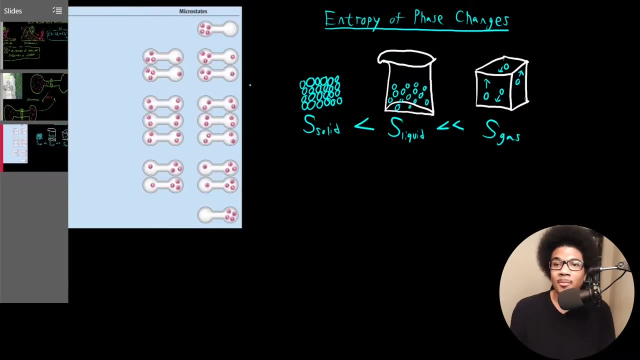 bulb Versus. if you just open it up and make all the space available to it, the gas is going to expand to fill that entire volume, right? So that would be the spontaneous process of gases expanding, right? So, and let's think about it from another perspective, 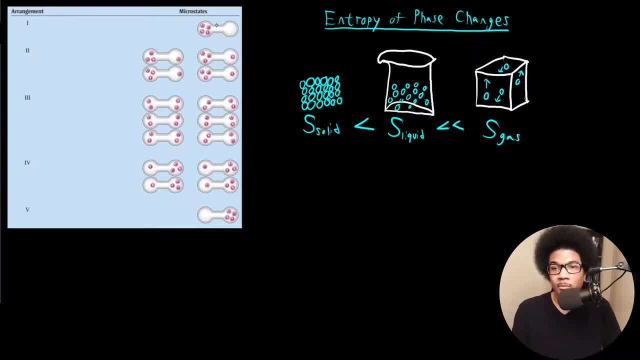 So let's take this two bulb system- the same two bulb system we've been working with or that we saw in the last one right- And let's say that, for example, there are four specific gas molecules In this two bulb system. we got a molecule- A, B, C and D, right? 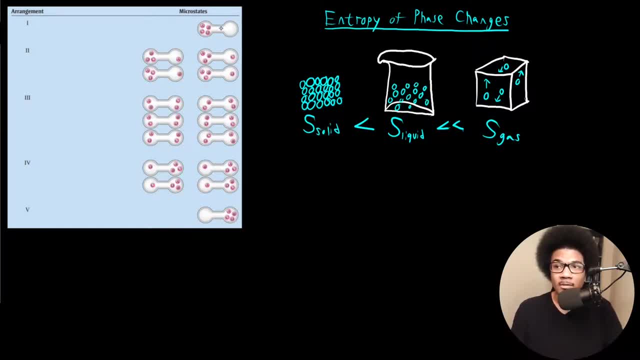 These four gas particles make up our entire system. If we think about it in this way, then we can think of five different ways that we could arrange these gas particles. We could have one arrangement where all of the gas particles are in the left bulb. 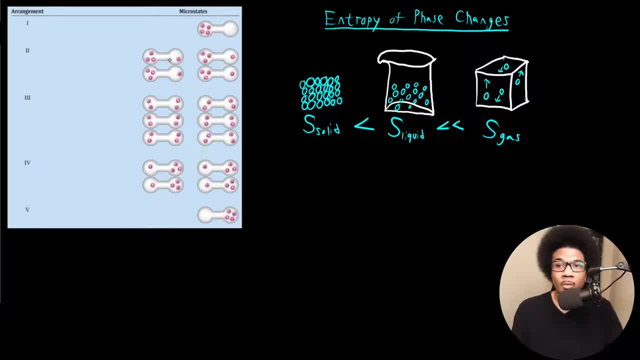 That's this arrangement one. We could have an arrangement where one gas particle is in the right bulb and the other three are in the left. We can have an arrangement where two gas particles are in the left bulb and two are in the right bulb. 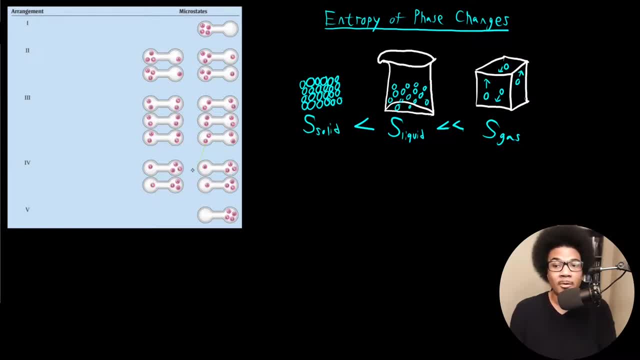 A fourth one where three are in the left right bulb and the one gas particle left is in the left bulb. And finally we can have one where all four gas particles are in the right bulb. Now what if I were to ask you if you were to pick one of these states at random? which? 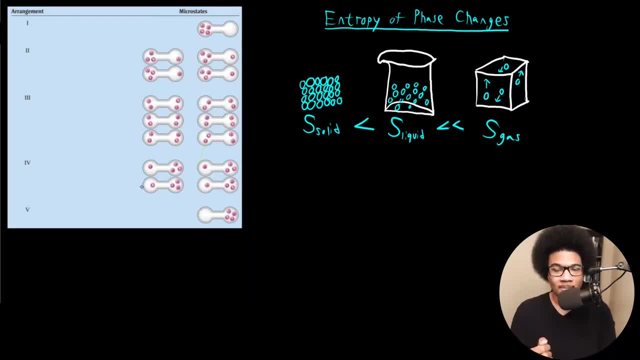 one are you most likely to pick? The answer here is going to be arrangement three: right. Why is that right? Why would you be most likely to pick if you were to pick one randomly? right, And just be able to stop the system and pick one at randomly? why would it be that you? 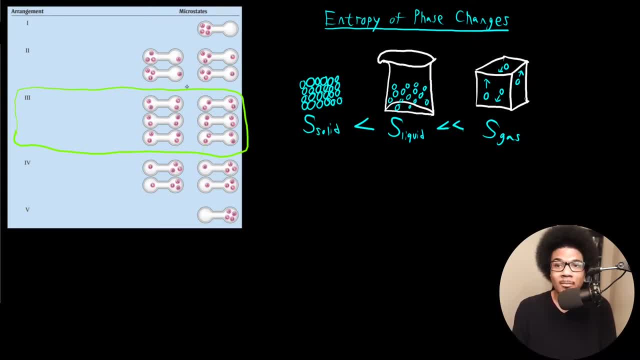 would pick one, most likely in arrangement three. Well, because it has the most possible states right. There's the most possible different ways that we can distribute these particles. exist where two particles are in the left and two particles on the right Right. 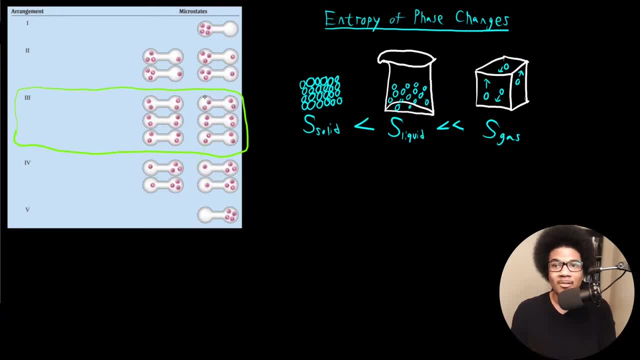 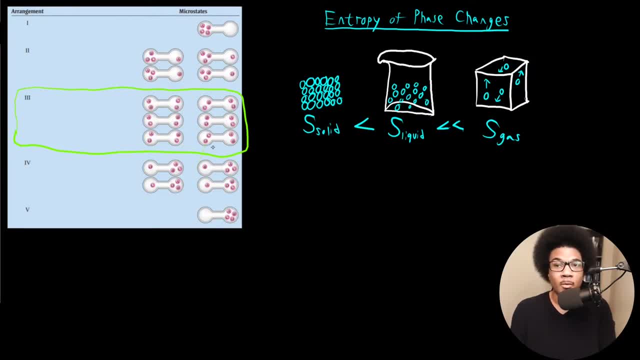 four and we only have one for arrangements one and four. It would be very unlikely to find the system in arrangement one or arrangement four Right. So this is how nature works, right? Something that is more disordered right is more likely, right. 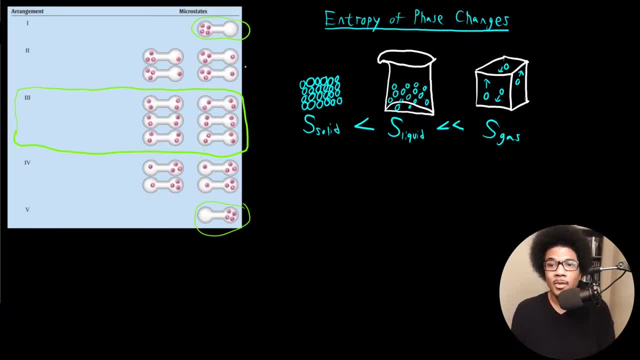 Something that is spontaneous is likely to occur, right, So you can kind of Glean a little bit of a qualitative understanding of why entropy and spontaneity have this link, just from looking at what is likely and what you know has more disorder associated with. 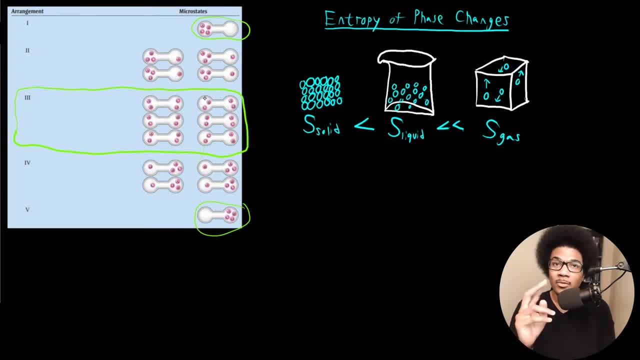 it Right. So, like I said, we'll make this link between spontaneity and entropy very explicit in the next video. I just wanted to give you a little bit of insight here Now. the last thing I wanted to touch on in this video is the entropy associated with. 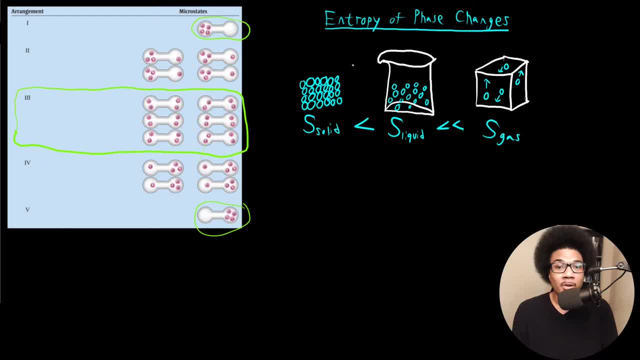 phase changes. Right, This will be the third phase of the universe, But if you're familiar with that, take a look at the にんじん and なんじん. Right, Because these are the three phases of matter. 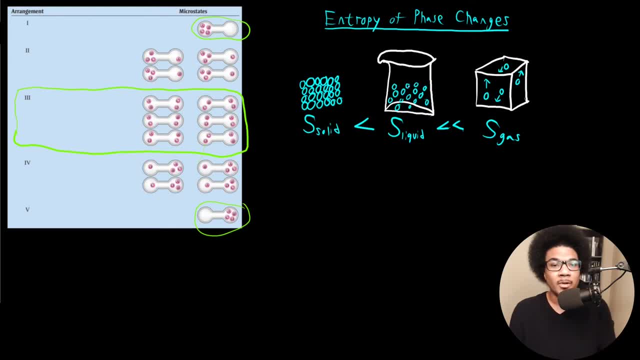 Our three main phases of matter are solid, liquid and gas, and they look very different on a molecular level. Right Solids are very tightly densely packed together. Liquids are relatively densely packed, but a little bit more loose than solids.